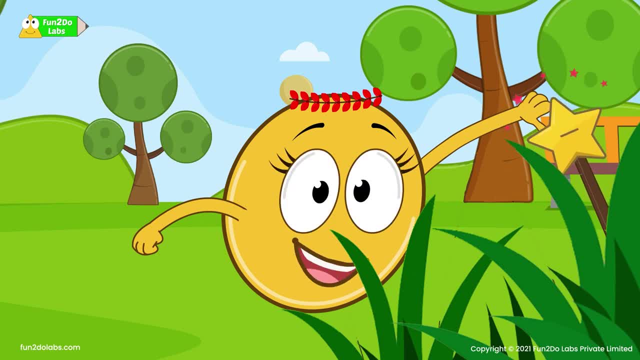 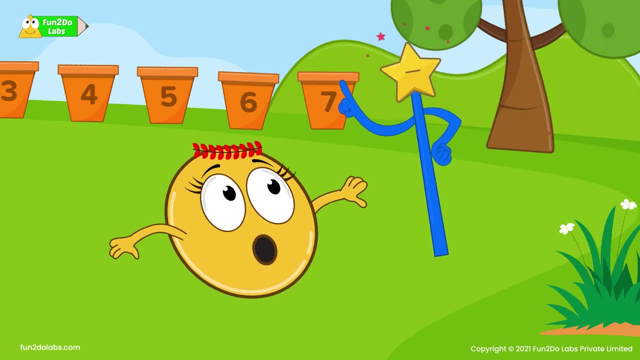 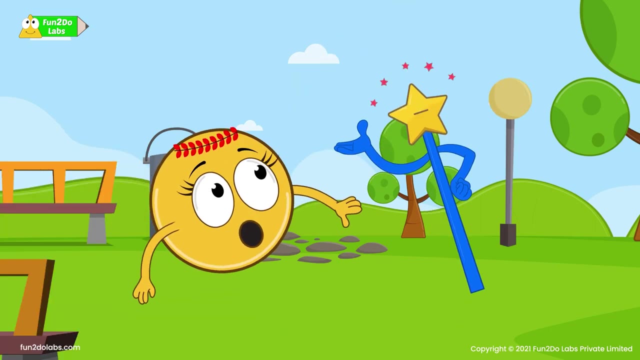 Wow, It looks like a gadget. Oh, I am, Ms Subtract, a mad gadget. I make things disappear by taking them away. Remember to make anything disappear. you need to tell me the correct answer of how many will remain in the end. 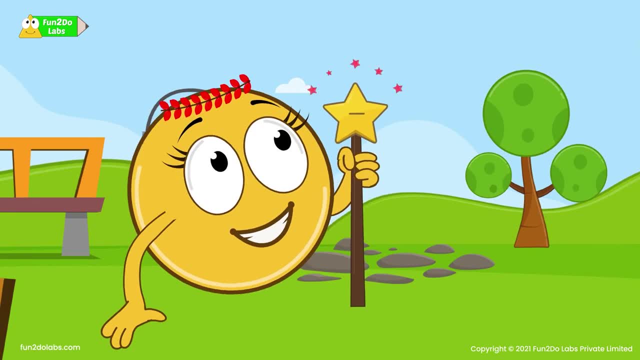 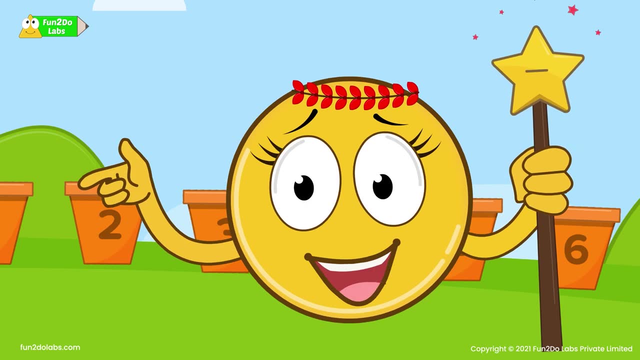 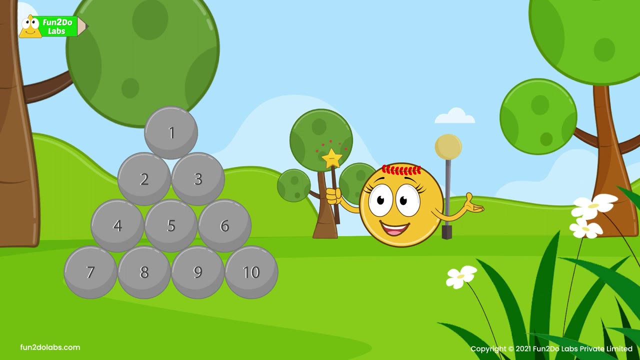 Sera always wanted to make things disappear without touching them. Now that I have Ms Subtract, I can fulfill my wish. Awesome, Let me try the gadget on some stones. first, Ms Subtract, take away six stones from the group of ten. 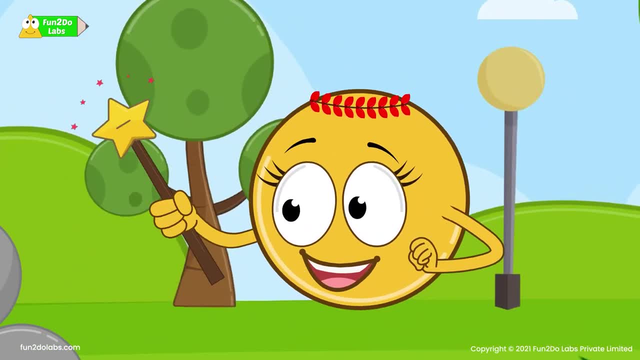 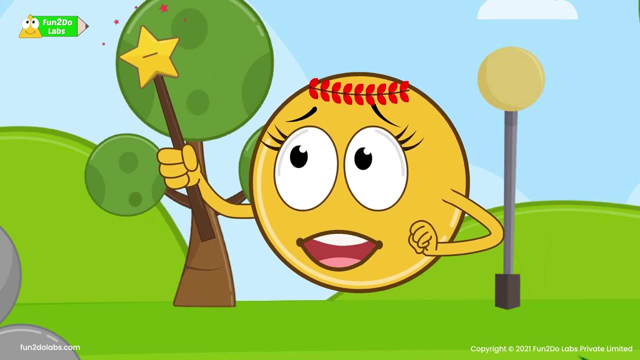 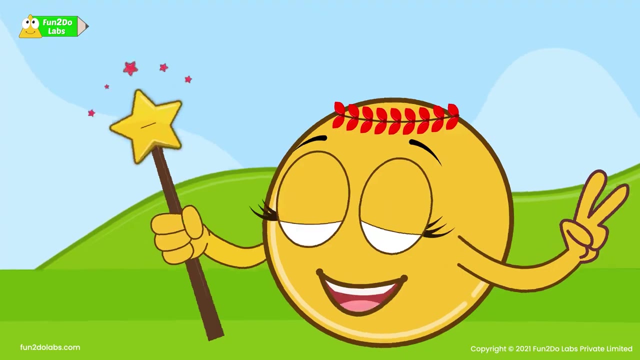 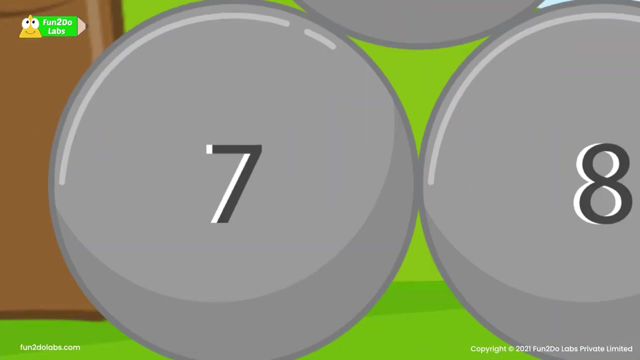 Only one stone remains, Go Go. Did the gadget really work? I guess no. Let me count the stones again to cross-check whether the gadget worked or not. What? One, two, three, four, five, six, seven, eight, nine, ten. 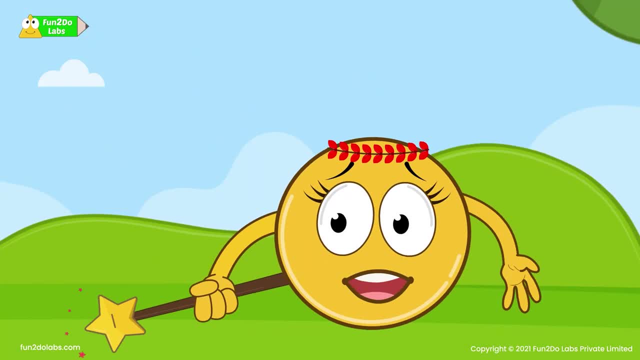 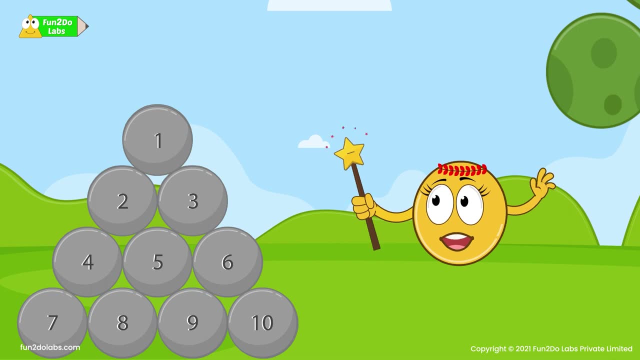 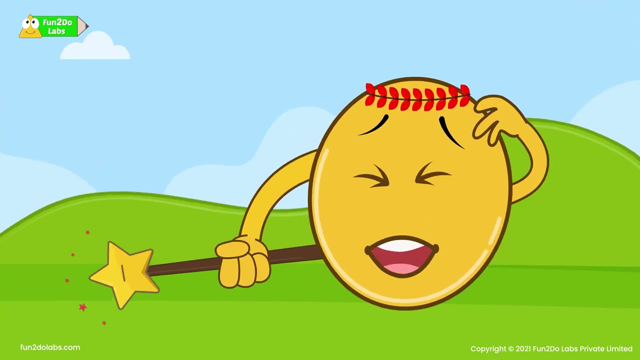 Oh no, They are still the same old ten stones. Sera does not give up. She tries again. Ms Subtract, take away six stones from the bunch of ten. Only two stones remain. Go. Oh no, The stones did not disappear. 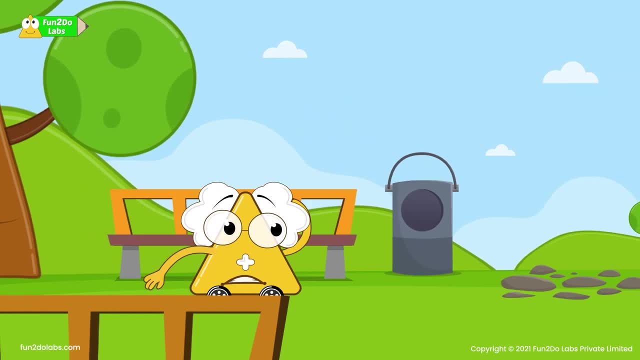 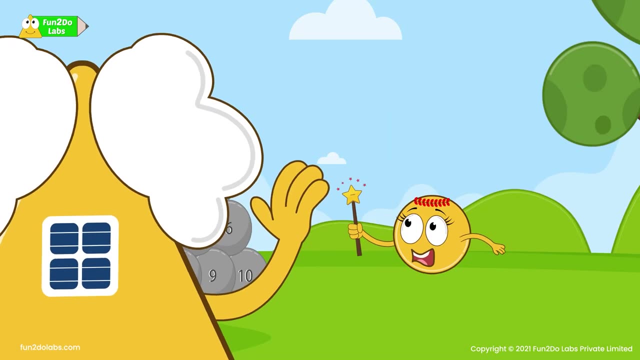 But why? Uncle Math is searching for something in the garden. Suddenly he spots Sera with the gadget, My gadget, My gadget. I have been looking for it since the morning. Where did you find it? I was playing in the morning. 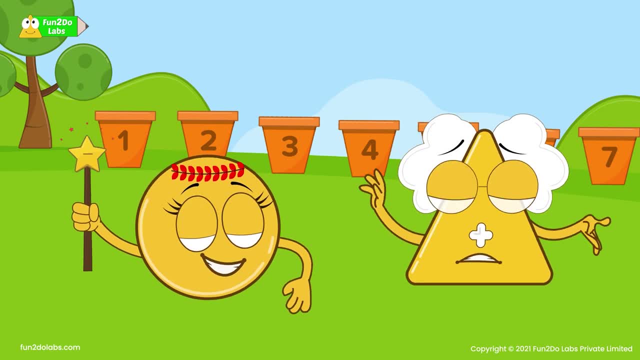 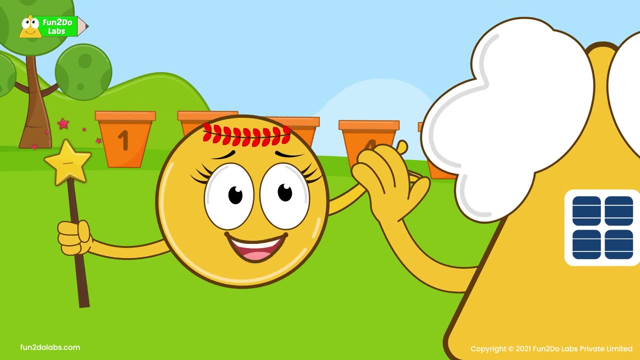 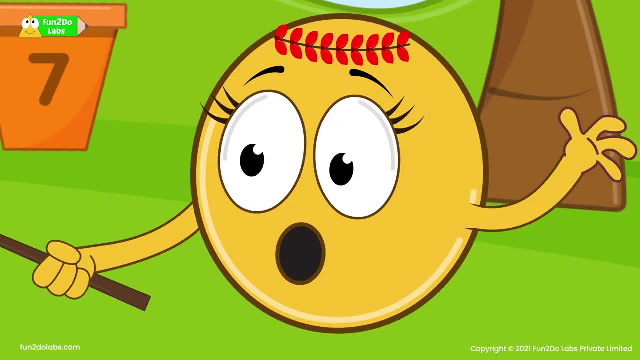 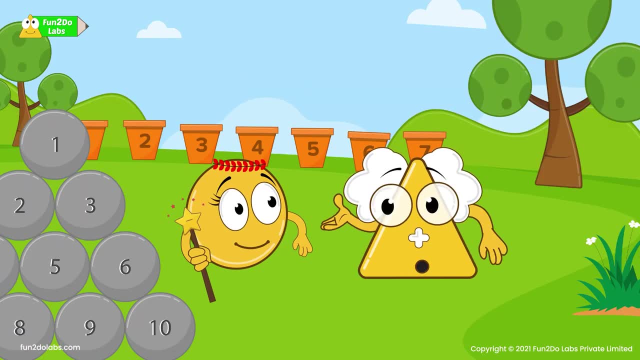 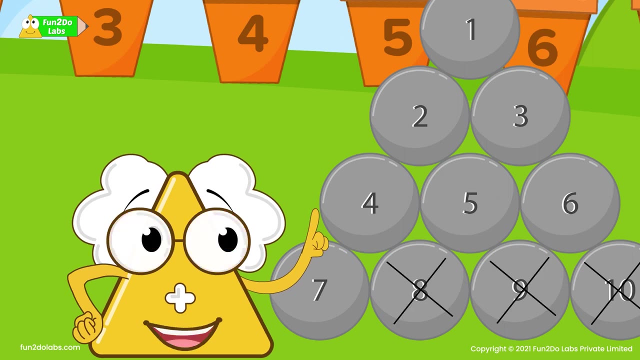 Oh, my And her struggles with the gadget. All right, I will help you, Sira. Miss Subtract is not working because your answer is wrong. See, here are your ten stones. If I take away six, how many remain? One, two, three, four. 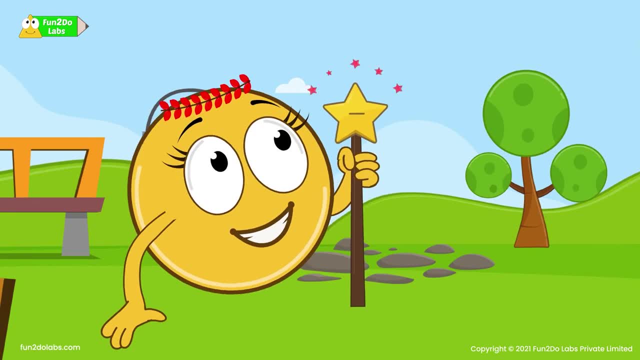 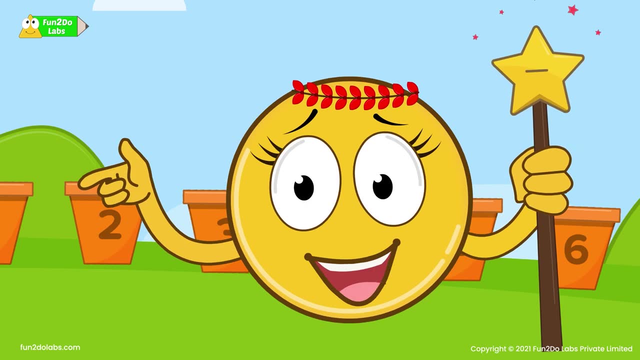 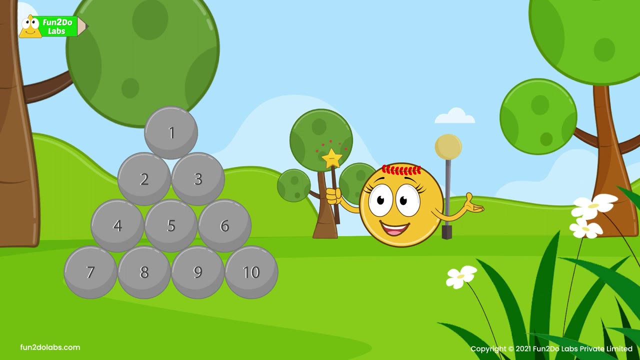 Sera always wanted to make things disappear without touching them. Now that I have Ms Subtract, I can fulfill my wish. Awesome, Let me try the gadget on some stones. first, Ms Subtract, take away six stones from the group of ten. 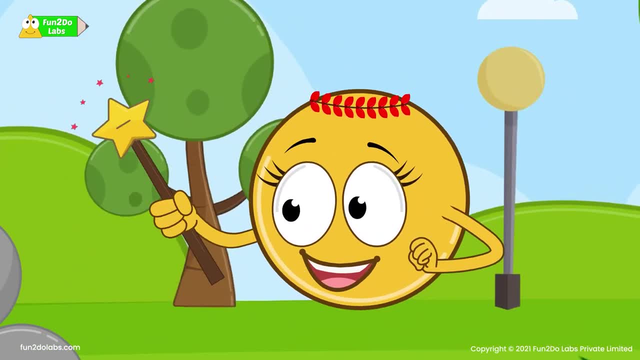 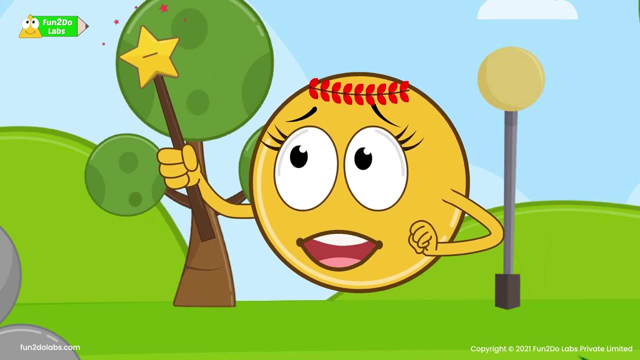 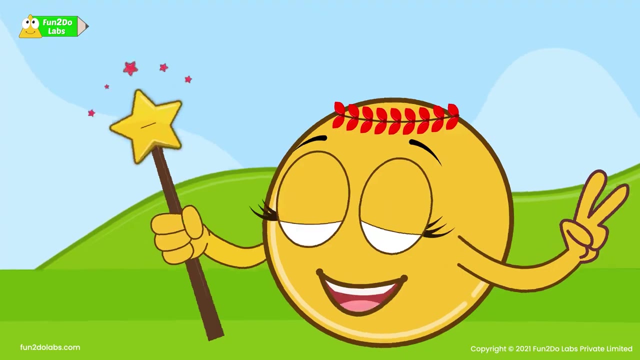 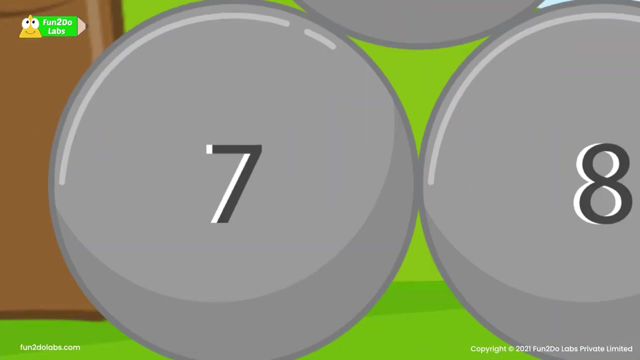 Only one stone remains, Go Go. Did the gadget really work? I guess no. Let me count the stones again to cross-check whether the gadget worked or not. What? One, two, three, four, five, six, seven, eight, nine, ten. 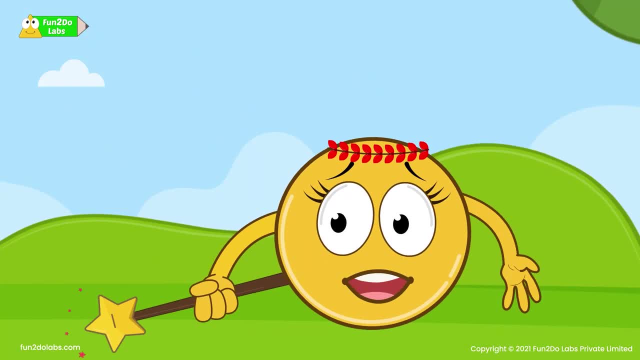 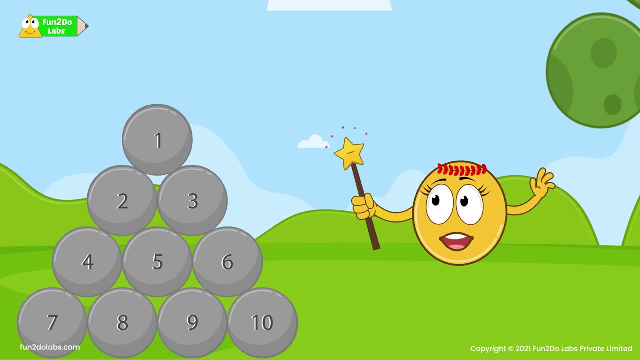 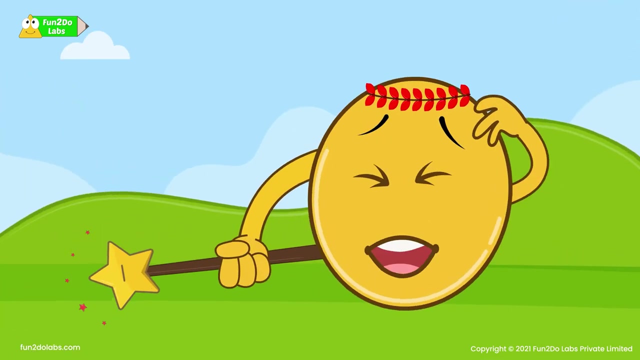 Oh no, They are still the same old ten stones. Sera does not give up. She tries again. Ms Subtract, take away six stones from the bunch of ten. Only two stones remain. Go. Oh no, The stones did not disappear. 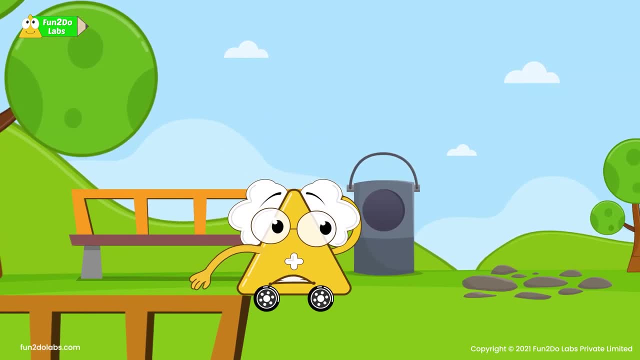 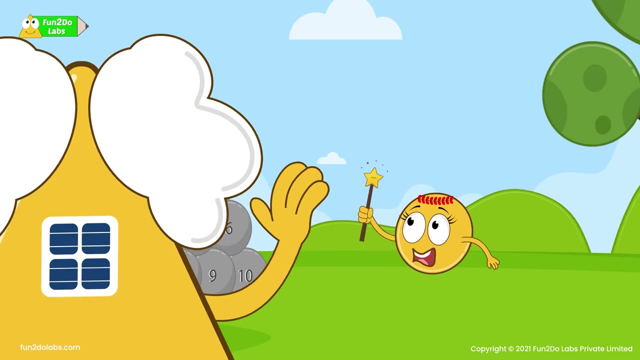 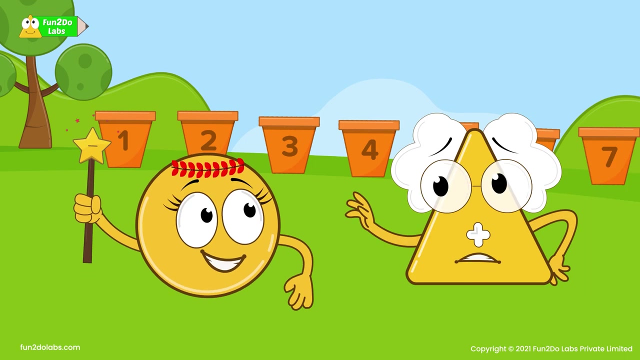 But why? Uncle Math is searching for something in the garden. Suddenly he spots Sera with the gadget, My gadget, my gadget. I have been looking for it since the morning. Where did you find it? I was playing in the morning. 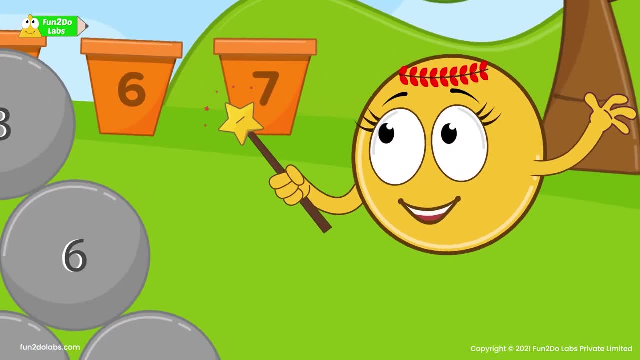 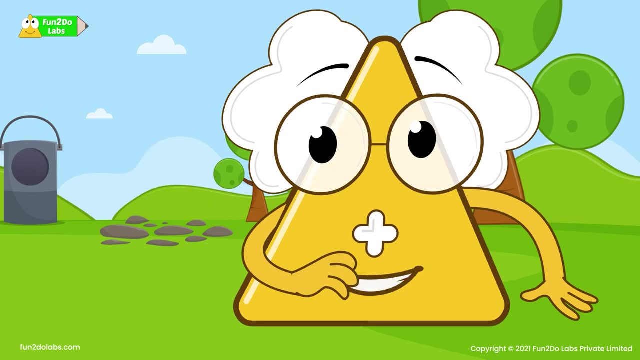 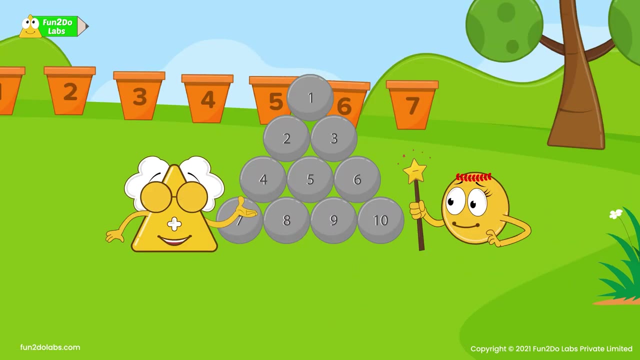 Sera quickly narrates the morning scene. Oh, She is excited because she has a steeply complicated knowledge of math. All right, I will help you, Sera. Ms Subtract is not working because your answer is wrong. Sera doesn't want to know the answer. 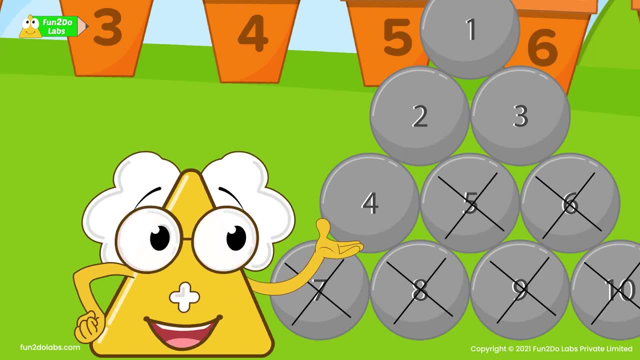 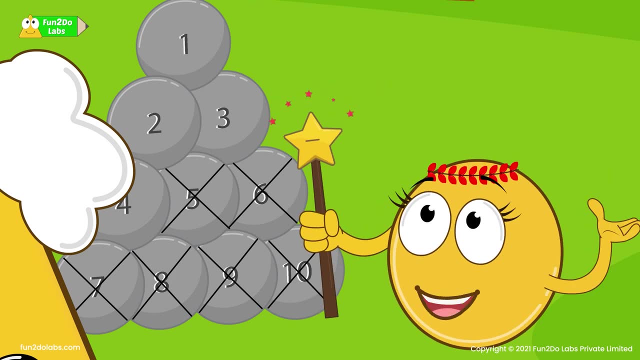 See, Here are your ten stones. If I take away six, how many remain? One, two, three, four, Four stones remain. Correct answer: Sera is becoming more and more angry. Sera is getting a lot forgettable. 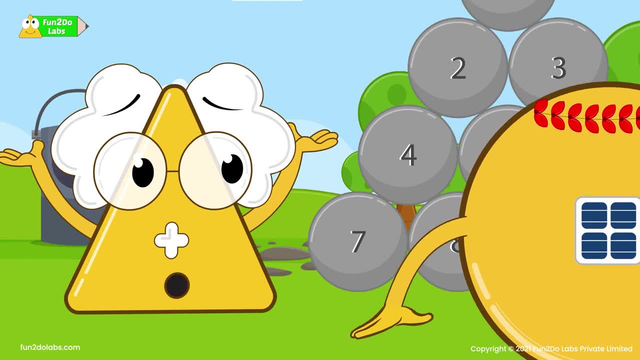 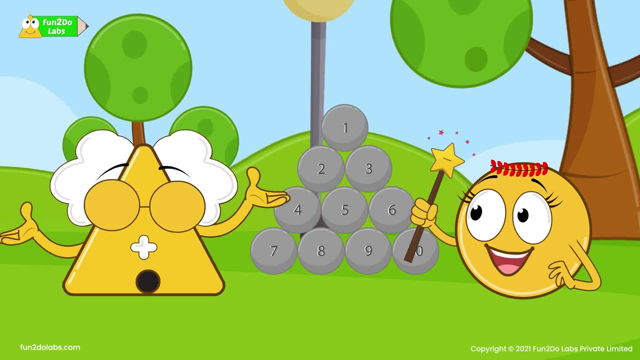 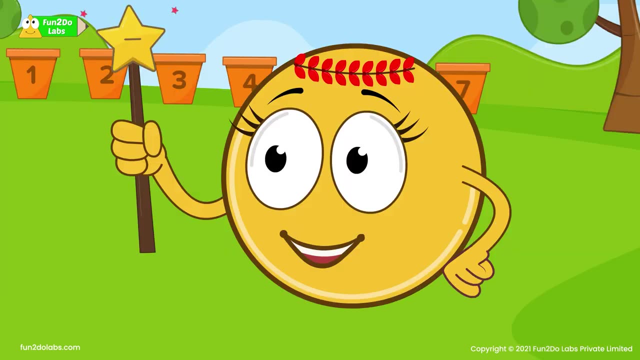 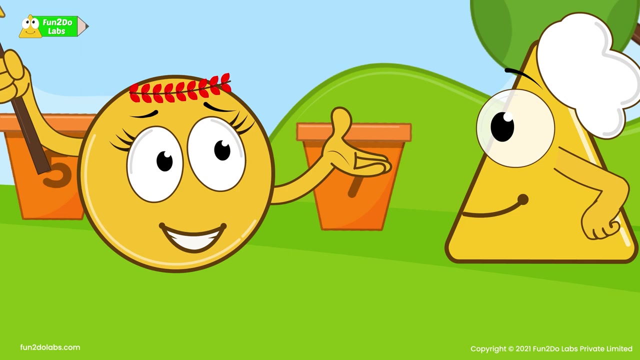 Taking away one or more things is called subtraction. We show subtraction using the minus symbol. So we say: ten stones minus six stones is equal to four stones. Oh, now I get it. I will use Ms Subtract on some pots now. 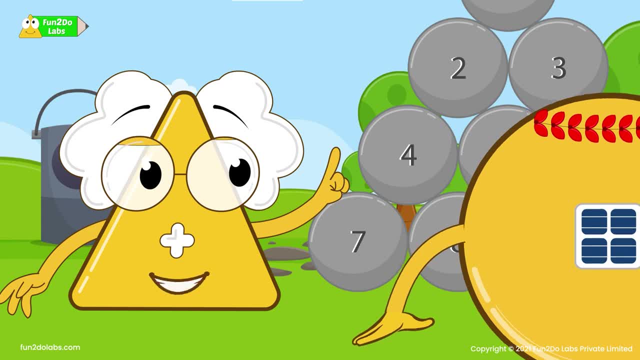 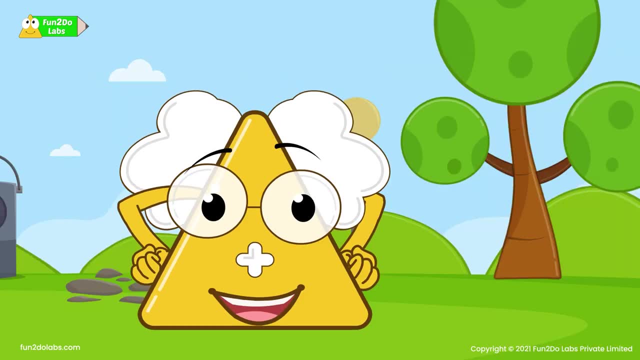 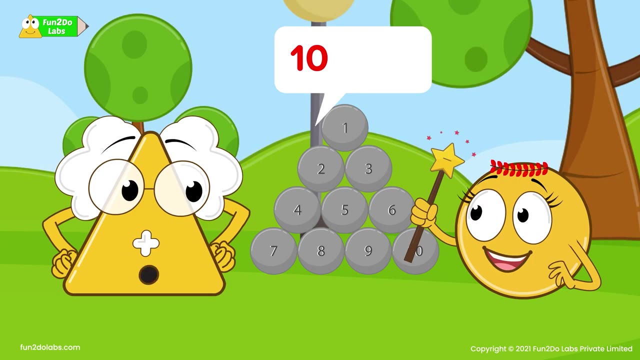 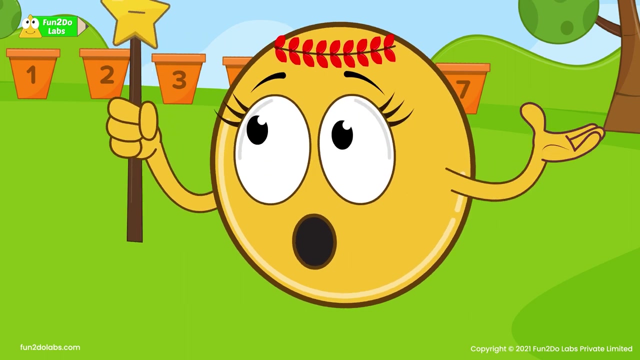 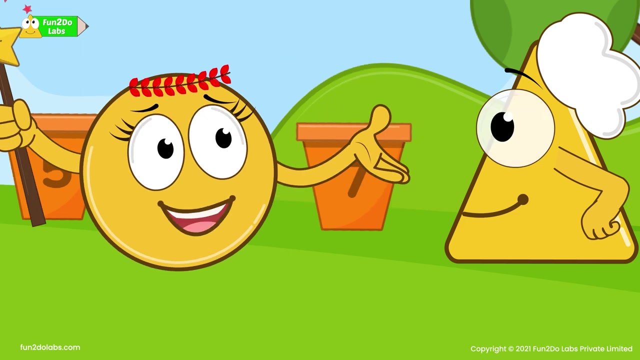 Four stones remain Correct answer. This method of taking away one or more things is called subtraction. We show subtraction using the minus symbol. So we say ten stones minus six stones is equal to four stones. Oh, now I get it. I will use Miss Subtract on some pots now. 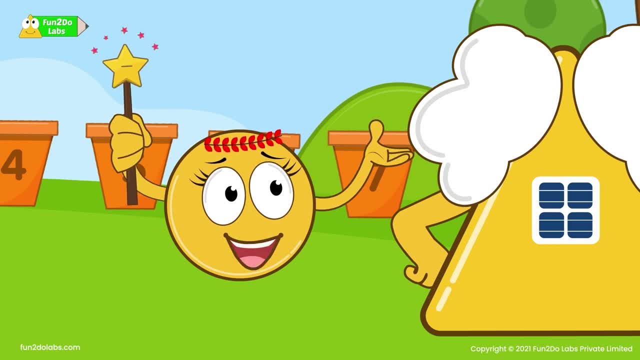 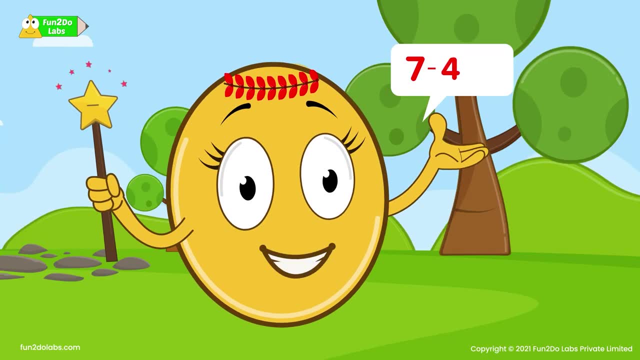 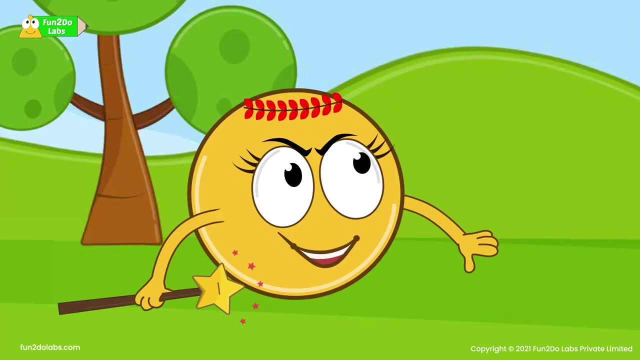 This time they will show. They will surely disappear. Uncle Math, Just wait and watch Miss Subtract take away four pots out of seven. Only three remain. Go Woohoo, I did it. Yes, you did it. Well done, Sira. 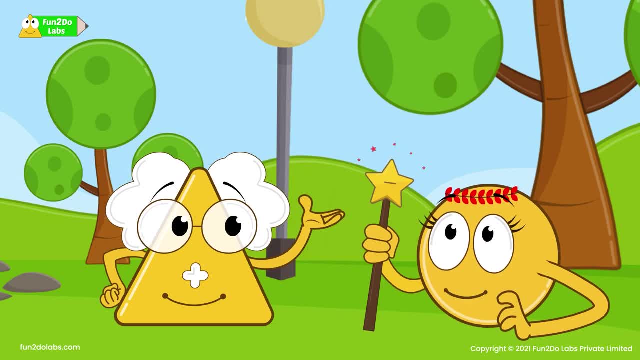 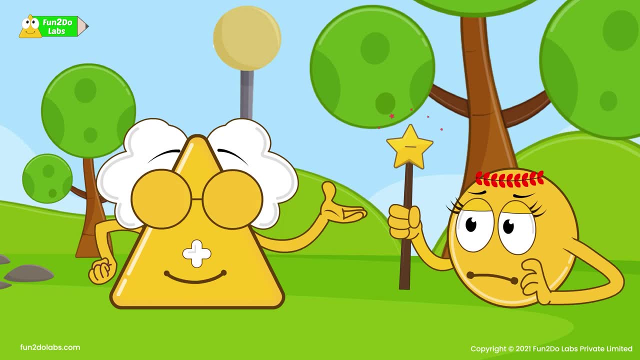 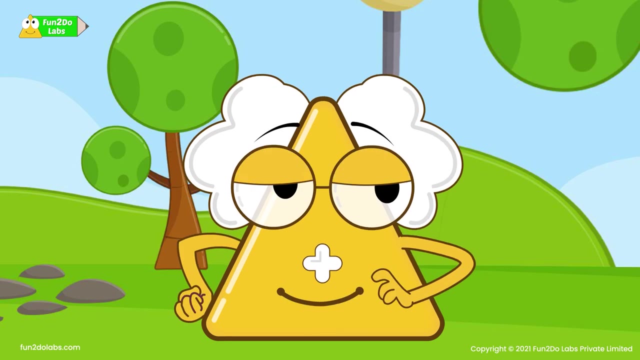 Let's make people disappear. now, Come on, What People? No, I might get hurt. How can I hurt anyone? I do not get you. If your gadget works, then everybody will like you. You will be famous. How is this hurting anyone? 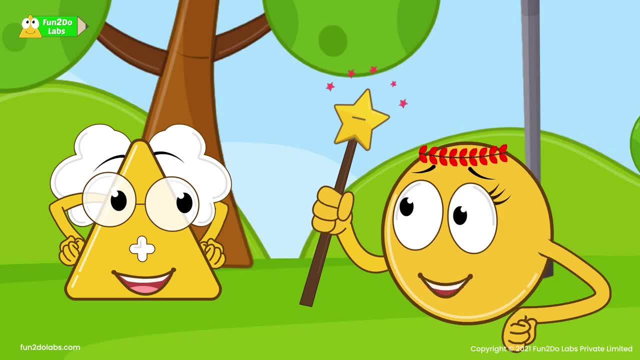 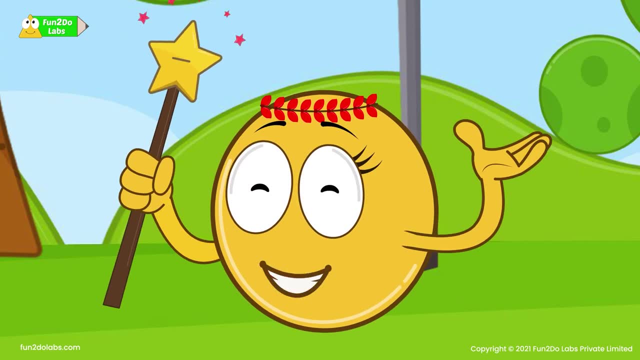 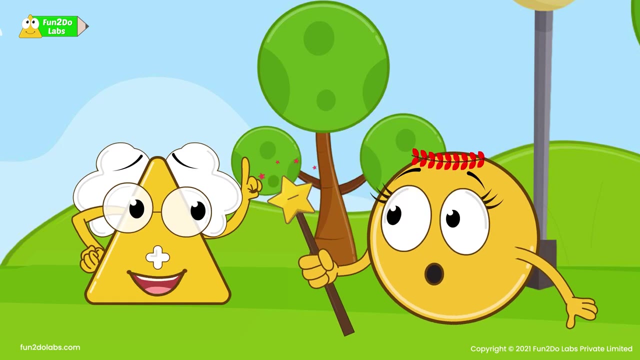 Definitely I will be famous, But if I try this gadget on innocent people for fun, then it would be selfish. I can't do this. Ha ha. I wanted to test you to see if you would misuse any of your superpowers. You might be less of an actor. 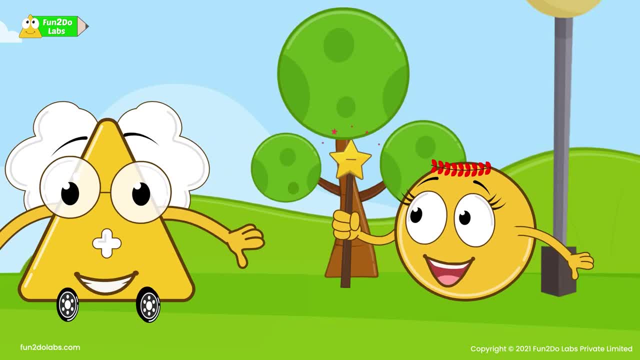 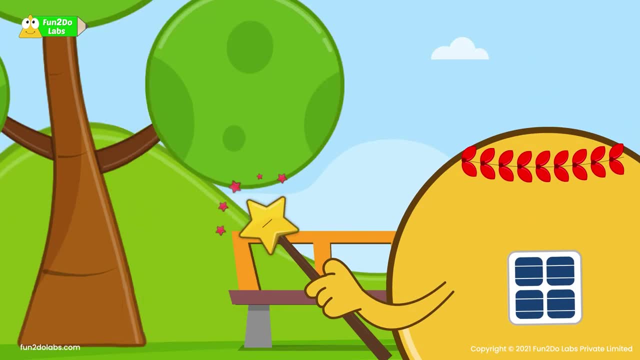 Ok, Get ready and go. Here is therente, And I got my answer. All right, I will leave now. See you A tube scope. When the gadget became Sira's superpower, she decided to use it only for learning, without hurting anyone. 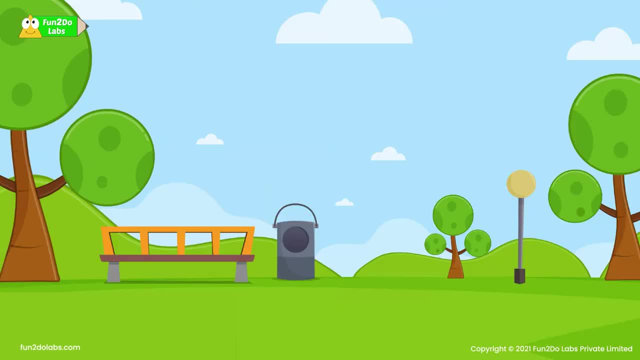 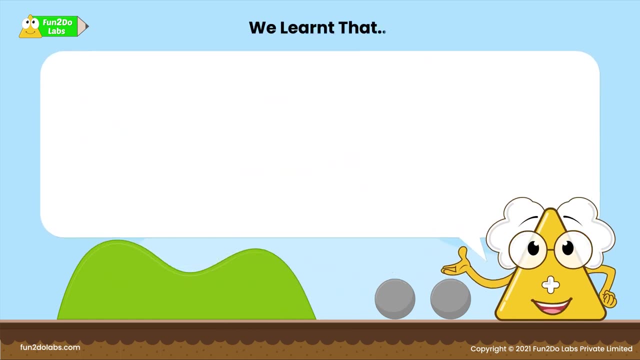 With great power comes great responsibility. Walt Disney made this ruler beautiful, Indeed, beautiful gesture, beautiful subtraction- obrai道ес- and beautiful Sira Cool. It is fantastic to see the result. eeny my, your oder. We learned that the method of taking away one or more things is called subtraction. 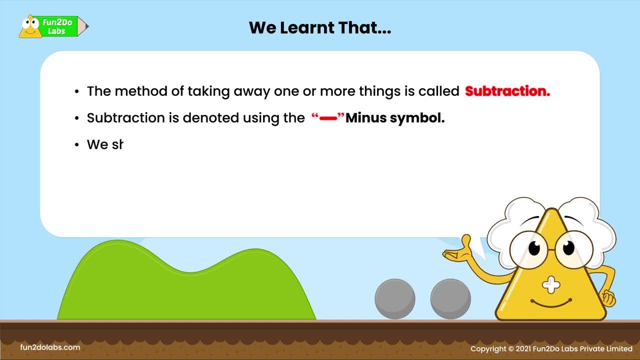 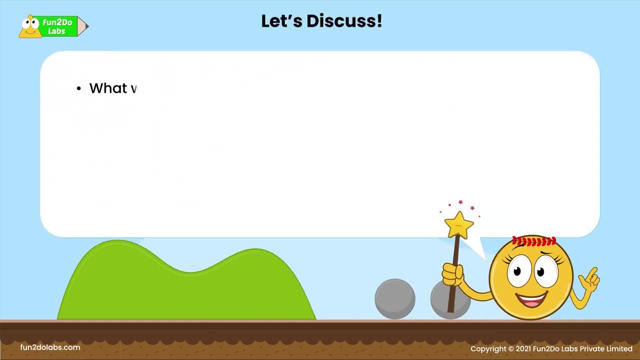 Subtraction is denoted using the minus symbol. We should never misuse our powers. We should not be selfish but empathetic towards others. With great power comes great responsibility. Let's discuss What was the name of the gadget. How did Uncle Math help me in using the gadget? 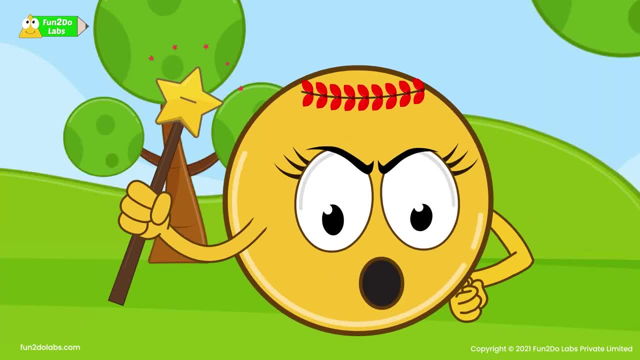 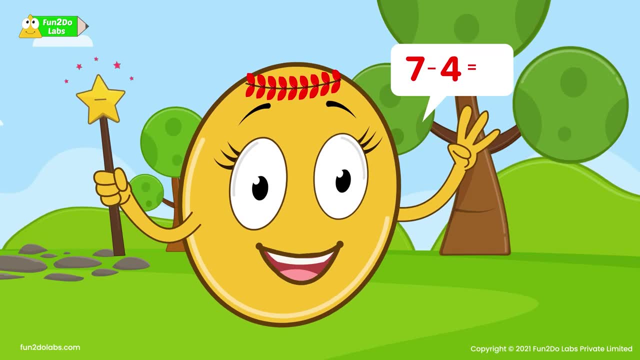 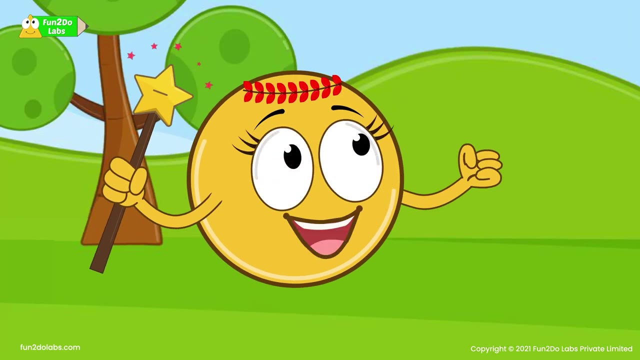 Next time they'll surely disappear. Uncle Math, Just wait and watch Ms Subtract take away four pots out of seven. Only three remain. Go Wahoo, I did it. Yes, you did it. Well done, Sira. 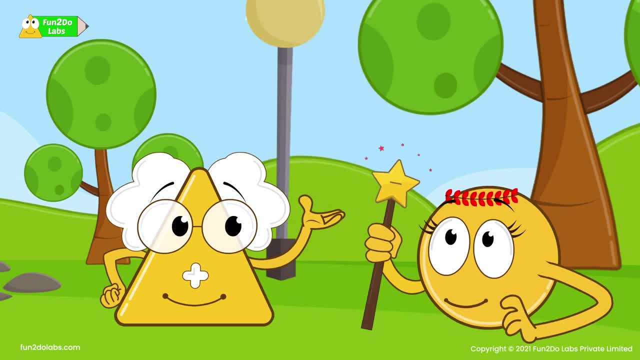 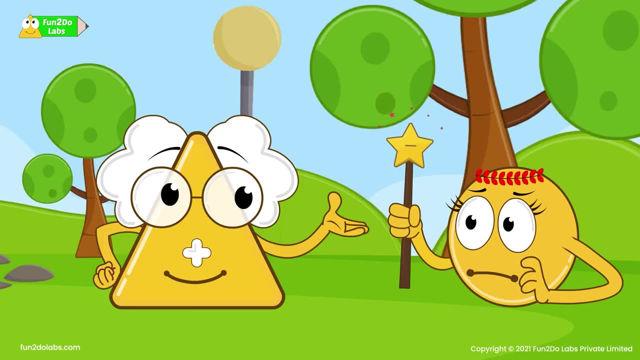 Let's make people disappear. now, Come on, What People? No, People must disappear. People might get hurt. How can I hurt anyone? I do not get you. If your gadget works, then everybody will like you. You will be famous. 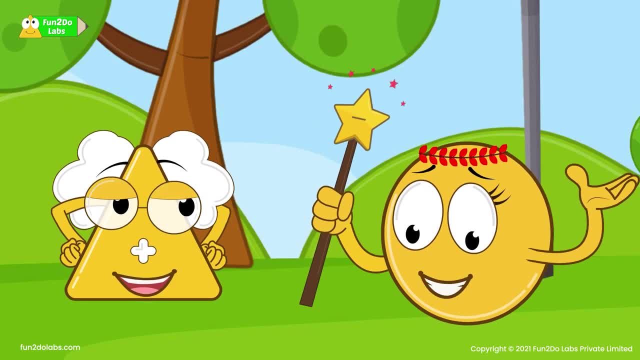 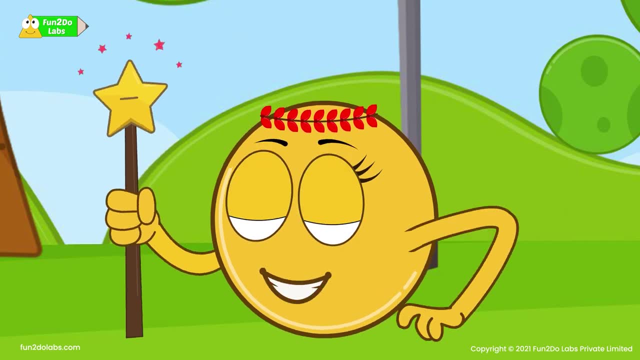 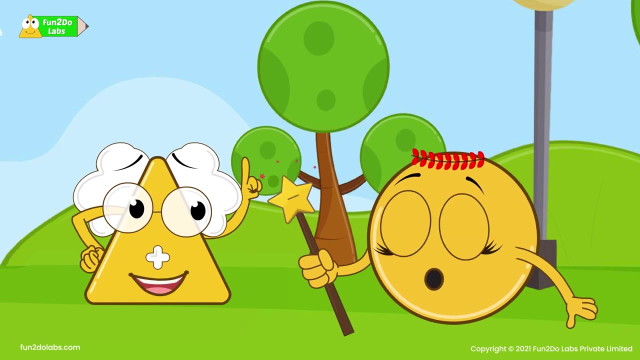 How is this hurting anyone? Definitely I will be famous, But if I try this gadget on innocent people for fun, then it would be selfish. I can't do this. I wanted to test you to see if you would misuse any of your superpowers. 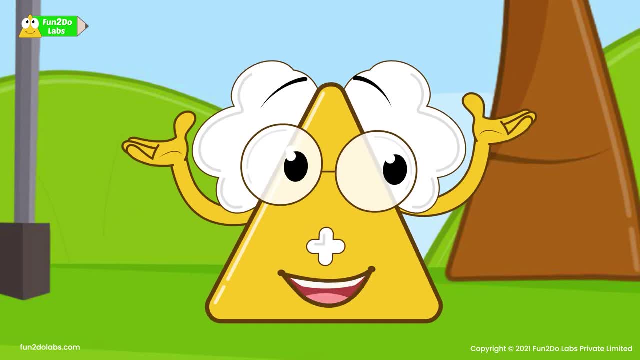 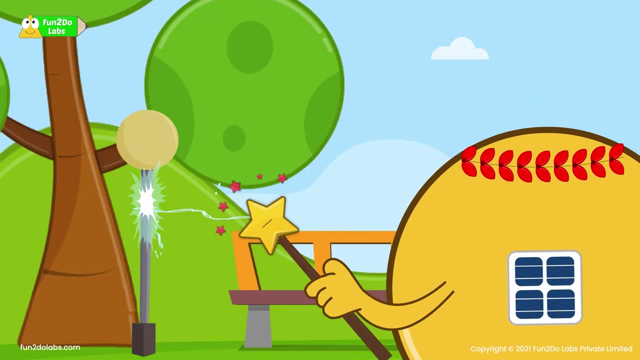 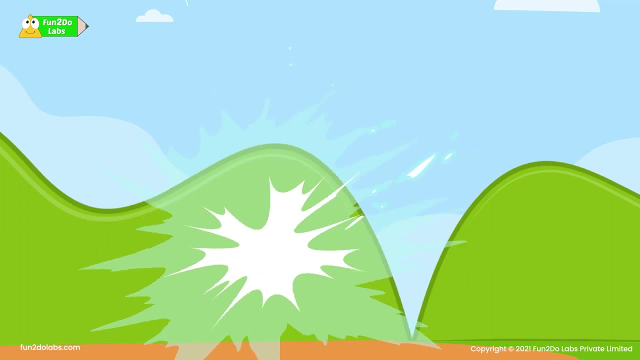 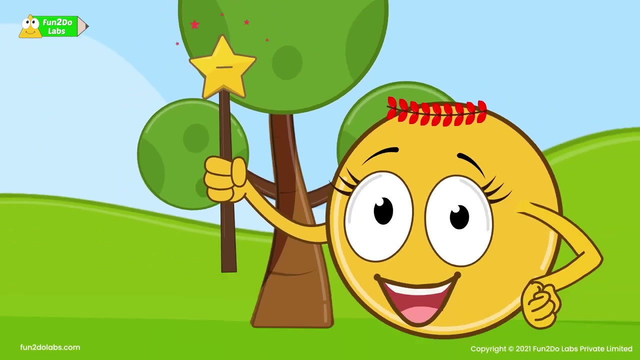 And I got my answer. Alright, I will leave now. See you, When the gadget became Sira's superpower, she decided to use it only for learning, without hurting anyone. With great power comes great responsibility. Indeed, beautiful gesture, beautiful subtraction and beautiful Sira. 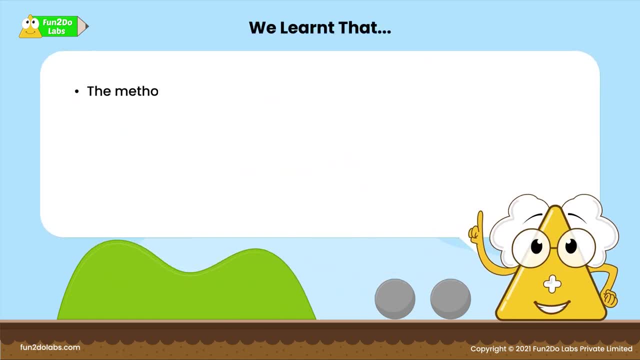 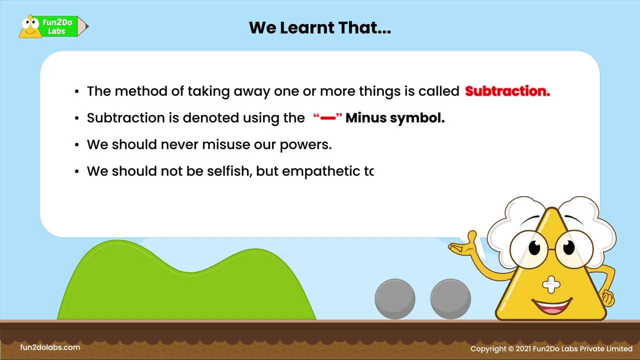 We learned that. Well done Bye. The method of taking away one or more things is called subtraction. Subtraction is denoted using the minus symbol. We should never misuse our powers. We should not be selfish but empathetic towards others. 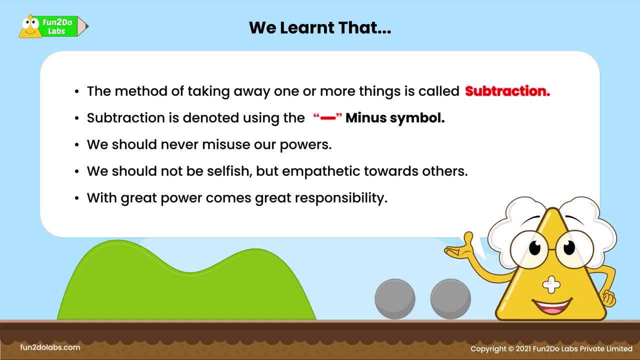 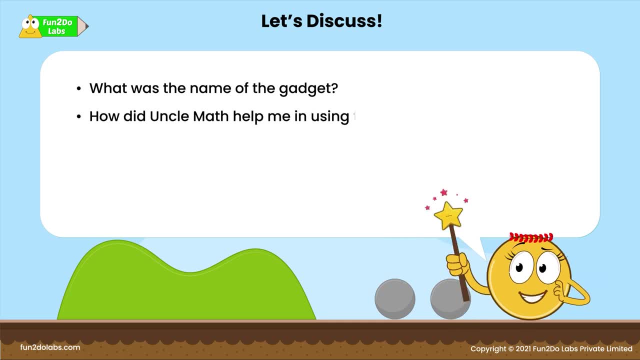 With great power comes great responsibility. Let's discuss. What was the name of the gadget. How did Uncle Math help me in using the gadget? I did not try the gadget on people. Is this good or bad? Why Explain? Miss Subtract became my superpower. 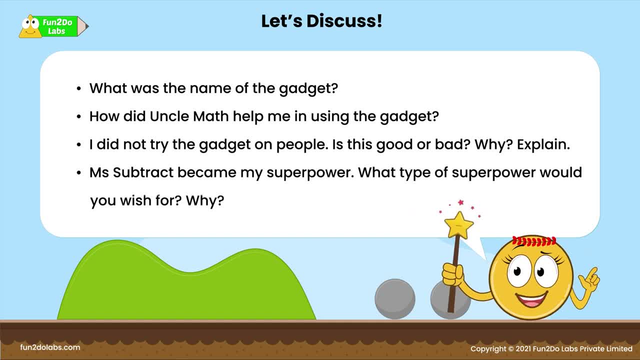 What type of superpower would you wish for? Why?